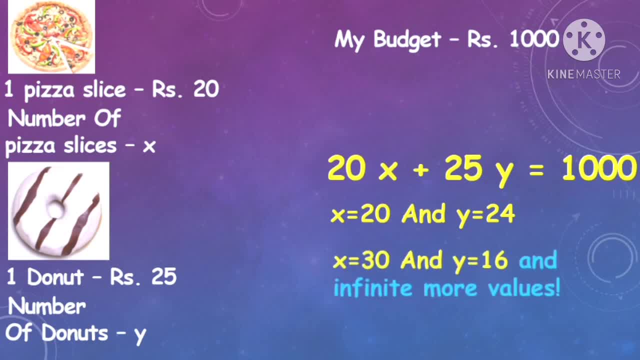 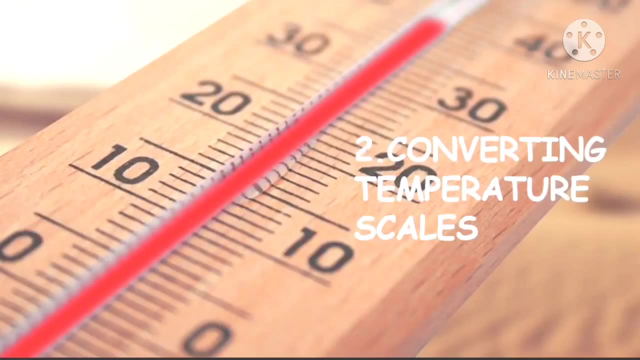 the number of pizzas. No problem, You can simply substitute, say, another value. I have taken x as 30 and I have got 16 donuts. There are infinite more possibilities, friends. So the next time you're hosting a party, you know who's help. to take The second application. 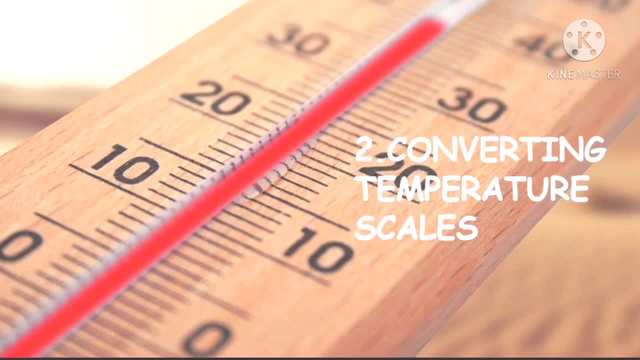 is temperature conversion. So, friends, recently I was in a call with a US friend who remarked that the temperature in his place was 95 degrees. Now I was shocked in the beginning, but then I realized that he was actually talking about the Fahrenheit scale. Now there is a. 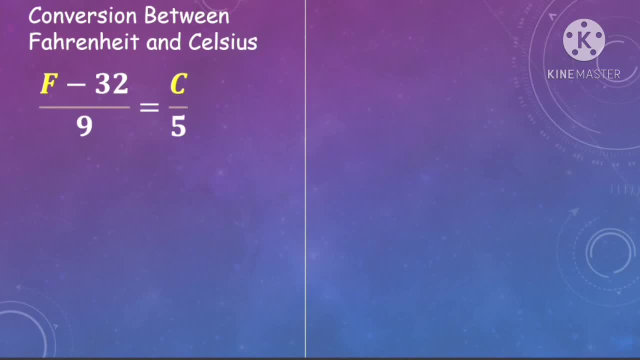 very simple linear equation that connects Fahrenheit and Celsius. F minus 32 upon 9 is equal to C upon 5, where F and C are the temperatures in Fahrenheit and Celsius respectively. So putting the value of 95 Fahrenheit and C upon 5,, that is the temperature in Fahrenheit. 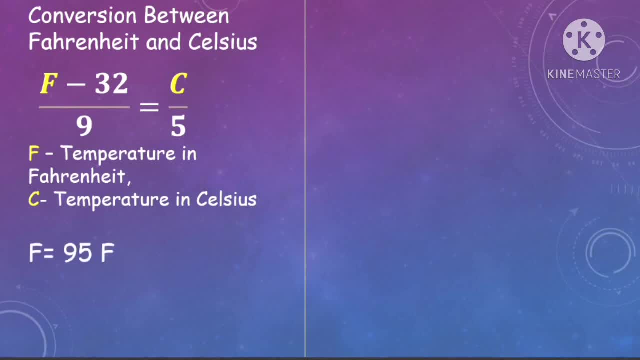 So putting the value of 95 Fahrenheit and C upon 5, that is the temperature in Fahrenheit, in my linear equation I actually got C to be 35 degrees Celsius, which is pretty normal. So if someone says it's 41 Fahrenheit, you can substitute in the linear equation and 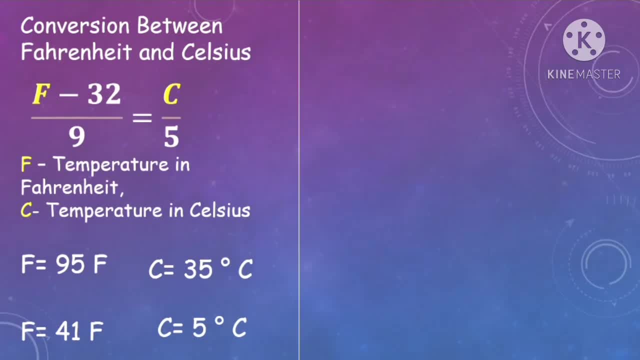 your value of C will be 5 degrees Celsius. Now there is another linear equation which connects Kelvin scale and Celsius scale. K is equal to C plus 273.. So you may ask: where is Kelvin scale used? Well, friends, it's made up of two things. The first one is that 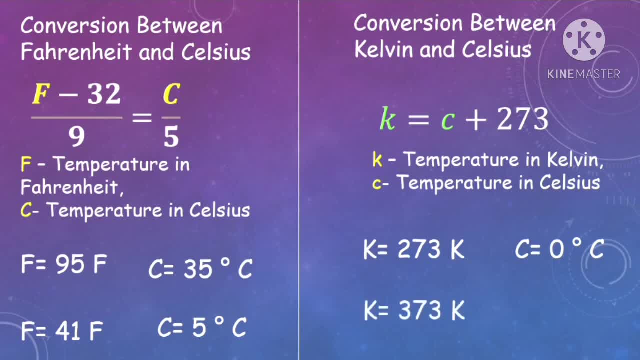 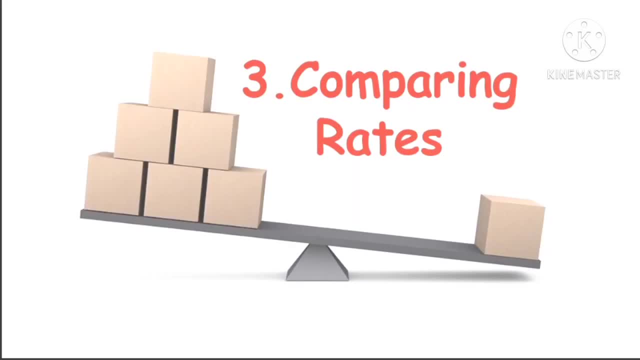 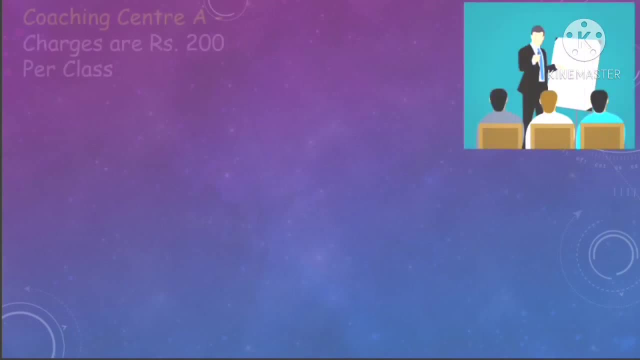 Kelvin scale is used in the lighting applications and also in photography, So this linear equation comes very handy indeed. The third application is comparing rates. So, friends, let's take the scenario of two coaching centers: Center A charges 200 rupees per class, whereas center 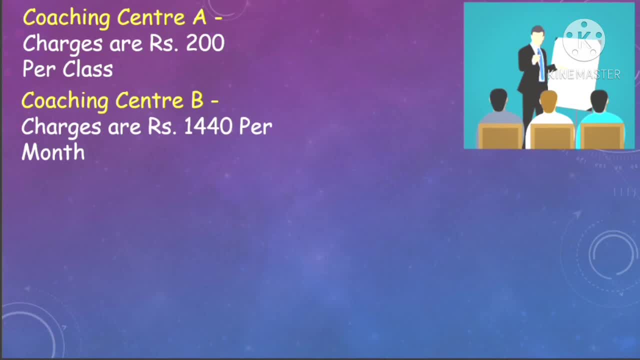 B charges 1440 per month. Both the centers take eight classes per month. We want to know which center is more affordable. So let's take the help of linear equations. Take X as the charge of center B for one class. We can make our own linear equation as 8X equal to 1440.. So on simplification we get. 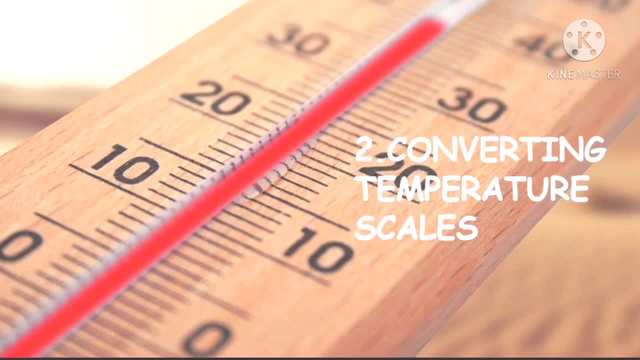 is temperature conversion. So, friends, recently I was in a call with a US friend who remarked that the temperature in his place was 95 degrees. Now I was shocked in the beginning, but then I realized that he was actually talking about the Fahrenheit scale. Now there is a. 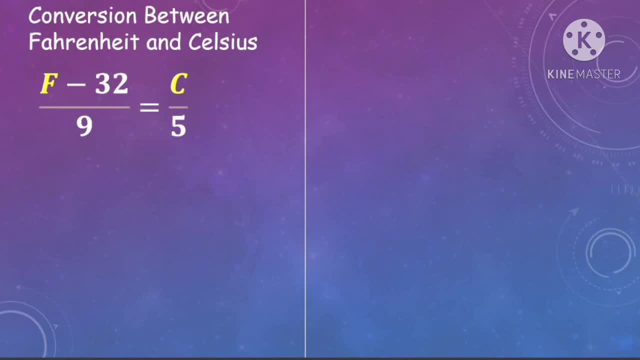 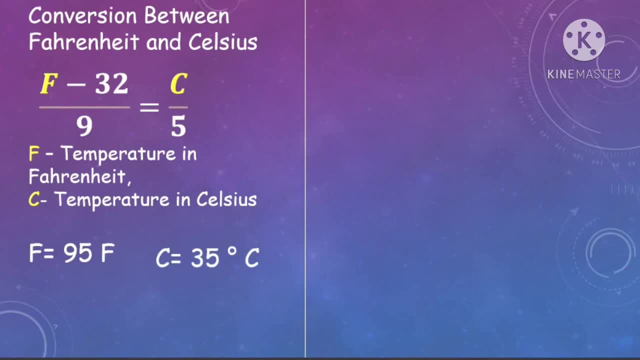 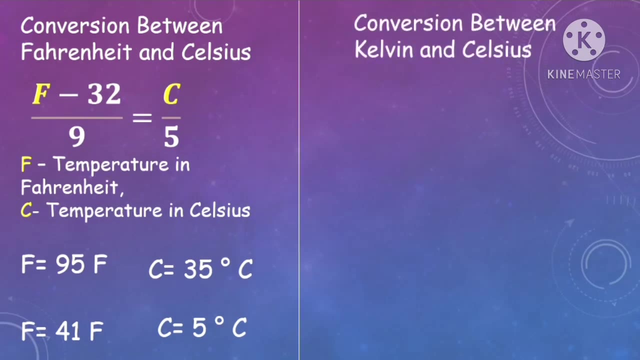 in my linear equation I actually got C to be 35 degrees Celsius, which is pretty normal. So someone says it's 41 Fahrenheit. You can substitute in the linear equation and your value of C will be five degrees Celsius. There is another linear equation which connects: 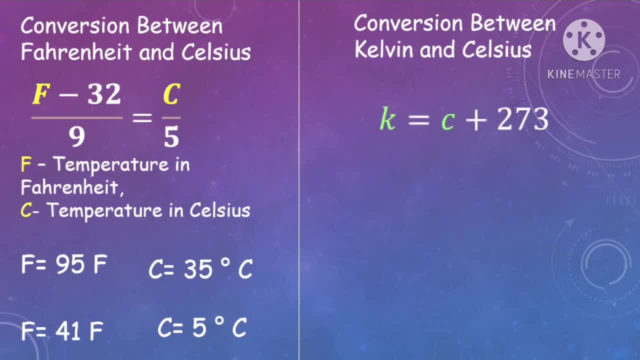 Kelvin scale and Celsius scale. K is equal to C plus 273.. So you may ask: where is Kelvin scale used? Well, friends, it's mainly related to the degree of concentration. So the number of degrees is a number minus minus. So we'll take that as K plus 273.. So you may ask where? 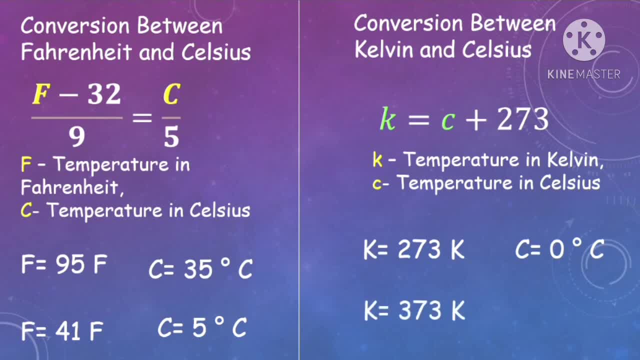 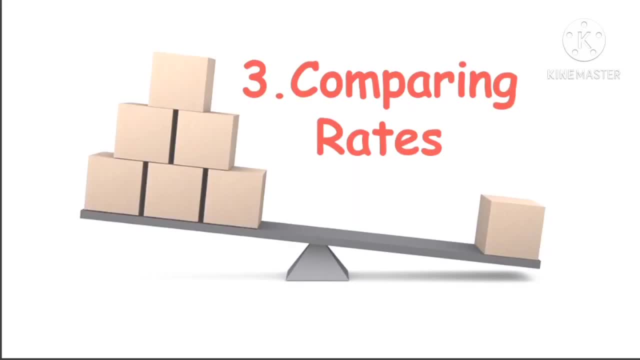 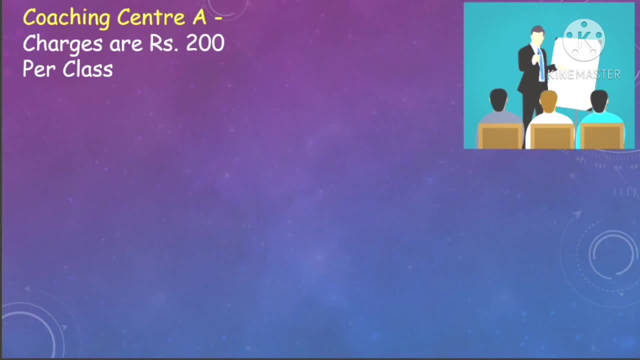 used in the lighting applications and also in photography. So this linear equation comes very handy indeed. The third application is comparing rates. So, friends, let's take the scenario of two coaching centres: Centre A charges 200 rupees per class, whereas Centre B charges. 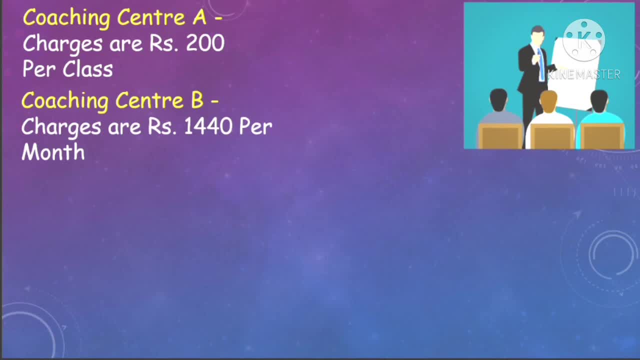 1440 per month. Both the centres take 8 classes per month. We want to know which centre is more affordable. So let's take the help of linear equations. Taking X as the charge of Centre B for one class, we can make our own linear equation as 8X equal to 1440.. So, on simplification. 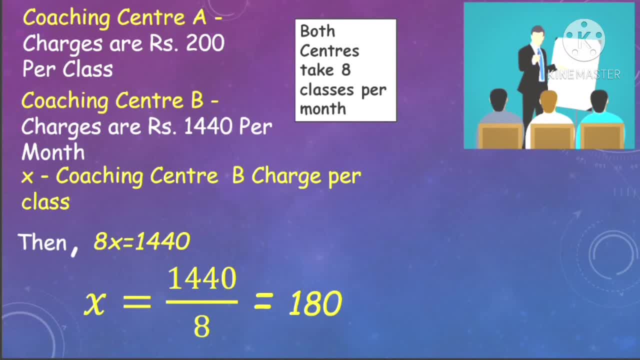 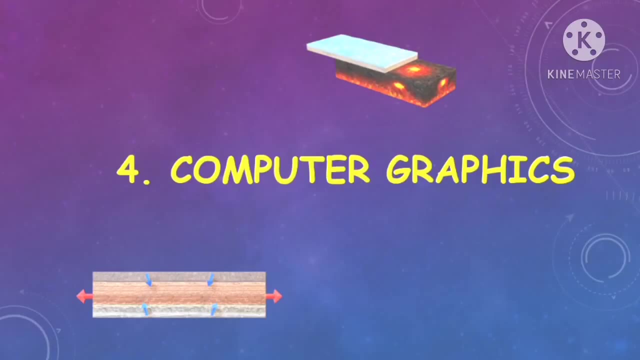 we get X is 180.. So Centre B charges rupees 180 only, which is much lesser than the charge of Centre A. So Centre B is obviously more affordable. So in this way linear equations are extremely helpful. The fourth application is computer graphics. Friends, did you know that a linear equation?